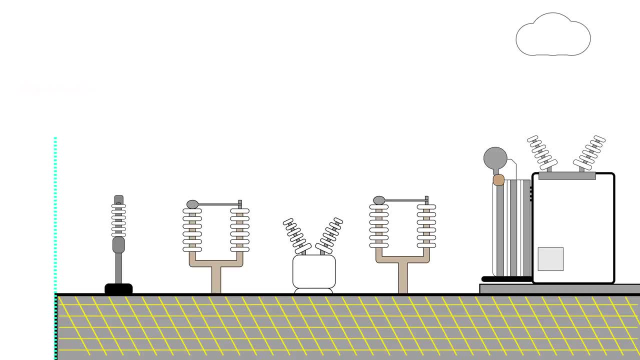 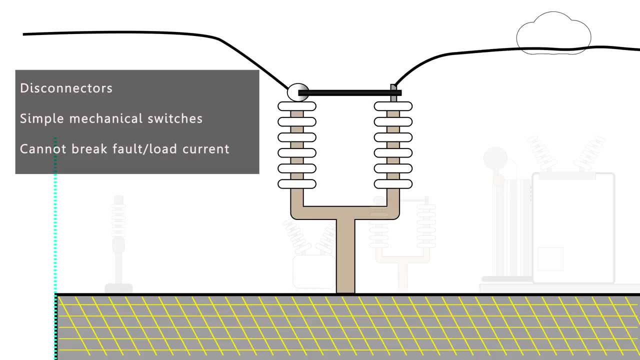 So the disconnector is a very simple asset in construction. It's made up of a swinging arm, So this is just really a mechanical switch. Now, disconnectors are cheap, They are reliable, but they're not able to break load current or fault current, So that's one of the big weaknesses of a disconnector. 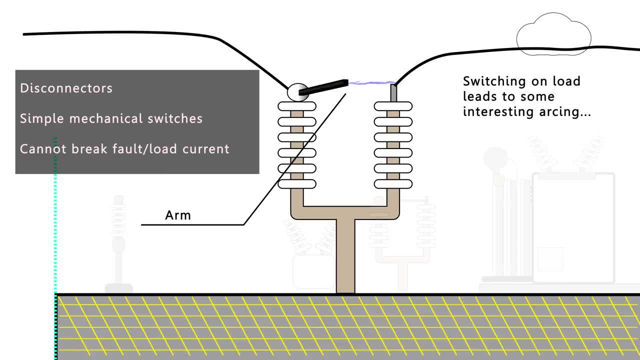 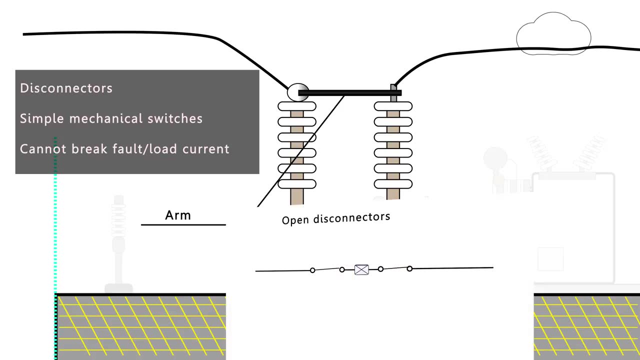 In fact if you try to break load current or fault current you just get a giant arc. So it's a very specialist job actually to break fault current and load current. But disconnectors do play an important role in the process. They play an important role inside the substation because they allow other assets. 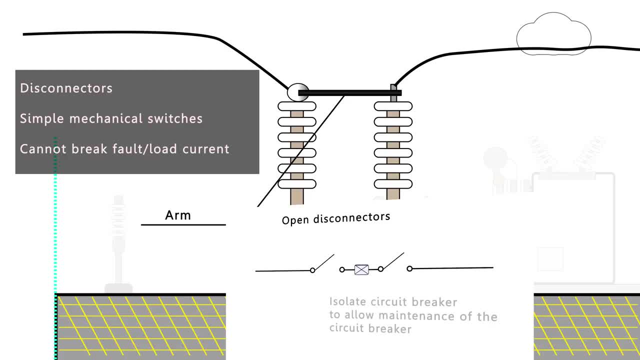 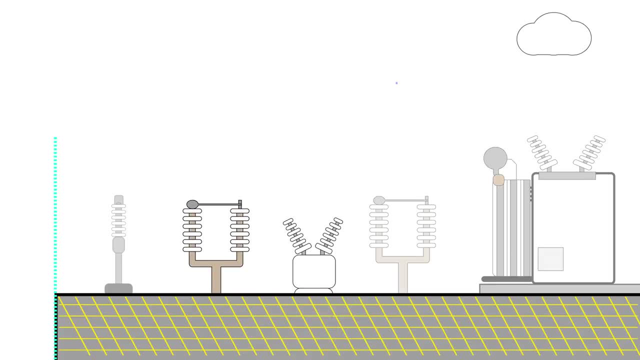 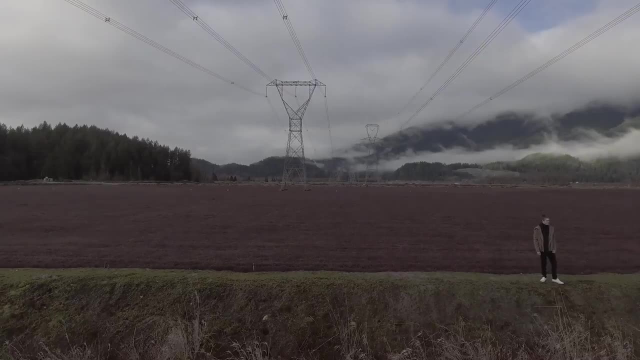 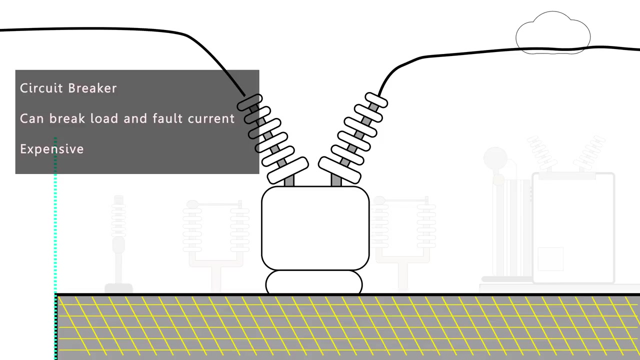 most importantly, the circuit breaker to be isolated. And it's reassuring if you're working or maintaining a circuit breaker, it's reassuring that you have that physical separation between you and the rest of the circuit That's a disconnector. Now we move on to the circuit breaker. So, as I mentioned before, the circuit breaker has the 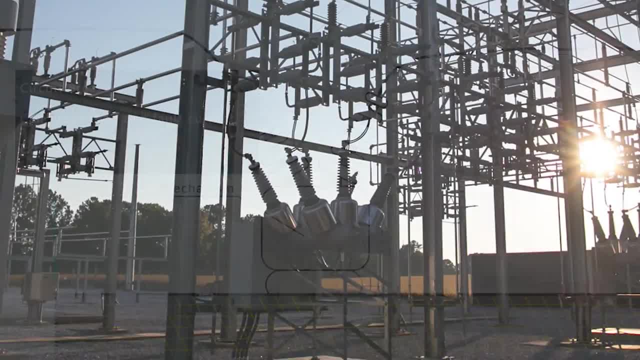 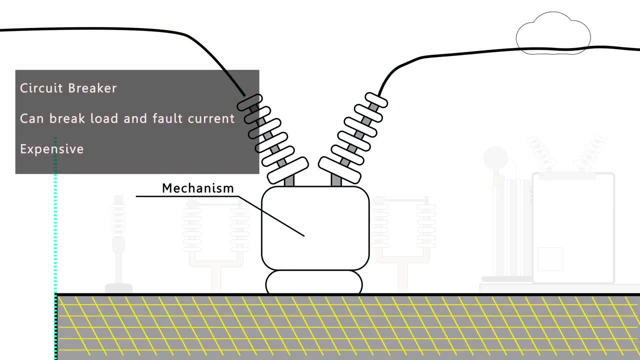 important and difficult job of breaking load current and fault current, And this is really difficult actually. So circuit breakers tend to be more complex in construction and therefore more expensive, but they play such a crucial role in the protection system of the substation. 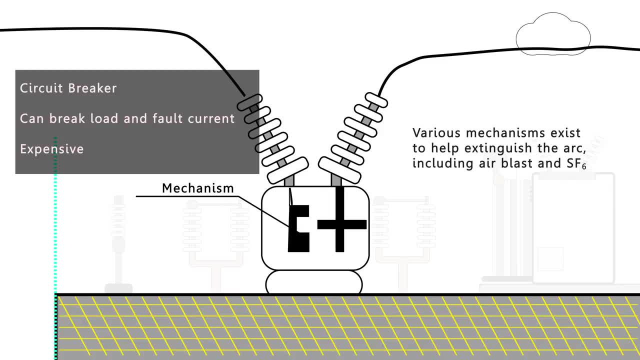 So most circuit breakers have some kind of mechanism to physically pull the two connections apart and then extinguish the arc. So examples of this are air blast circuit breakers and SF6 based circuit breakers. So that's the circuit breaker. They're very expensive but really important. 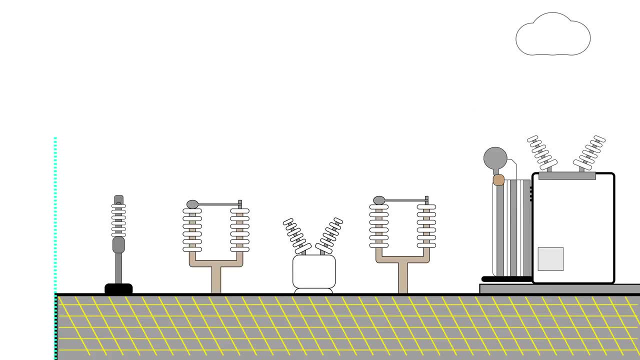 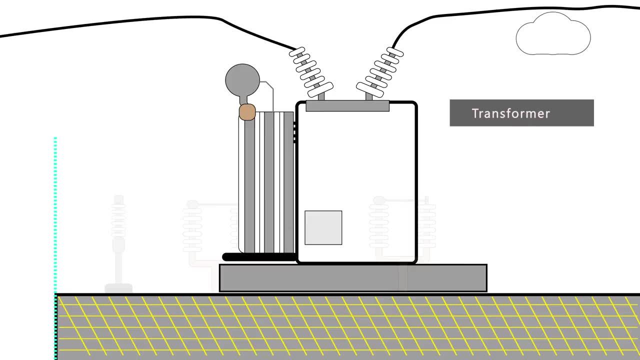 inside a substation. Now, the most expensive and largest asset inside the substation is the transformer. So the transformers really are playing a very important role inside a substation because the transformer is the biggest part of the system And it's the biggest part of the system. 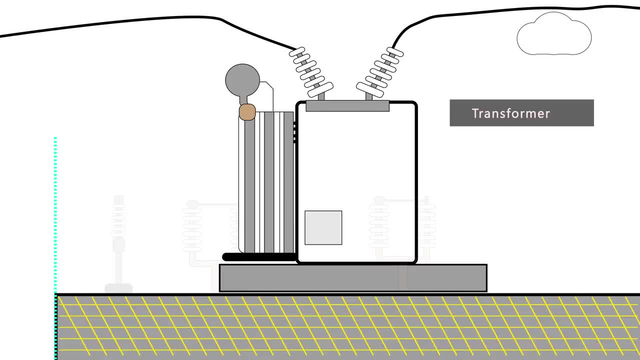 Now, one of the most striking features of the transformer is the giant radiator that's normally bolted on the side of the transformer. Now, the purpose of this radiator is to help with the cooling of the transformer, because, you know, transformers transfer vast amounts of energy and 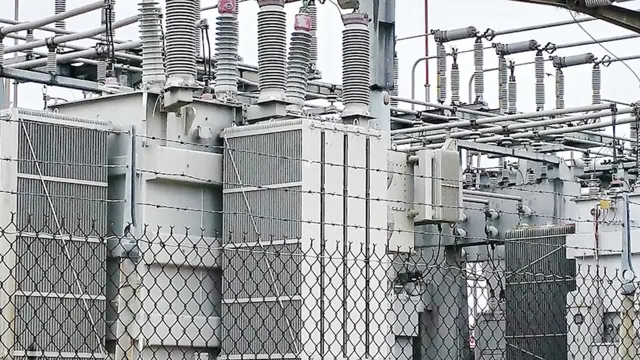 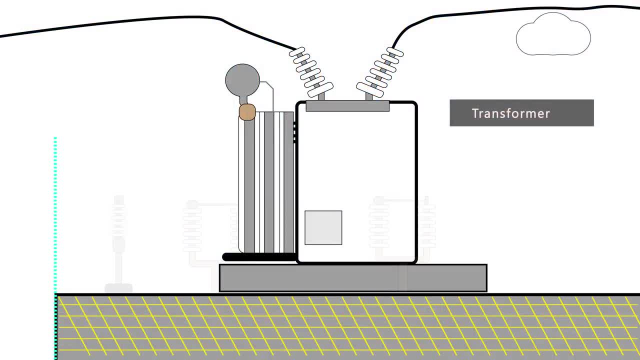 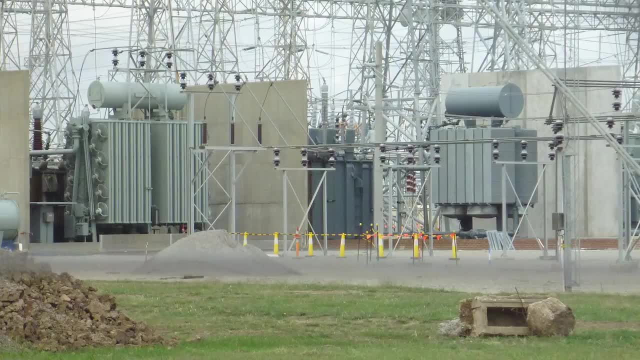 they do run hot, So oil is used as the coolant. But the radiator on the side is an additional measure to help cool down the transformer And typically oil will flow through the radiator and you'll have heat exchange. You also sometimes have fans underneath the radiator to 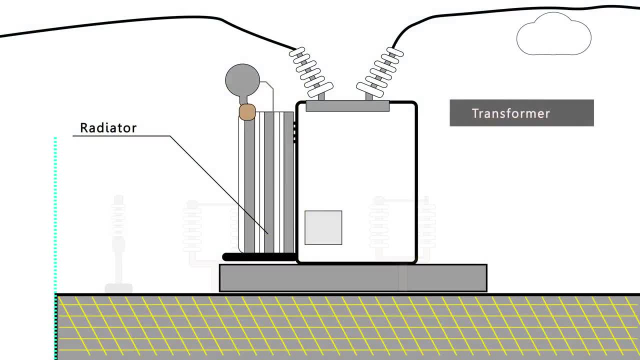 help with the cooling, just as you would in a laptop. actually, Now, the main chamber houses the windings And, of course, this is where the electrical role of the substate of the transformer is carried out: the stepping up and the stepping down- And we also have another. well, 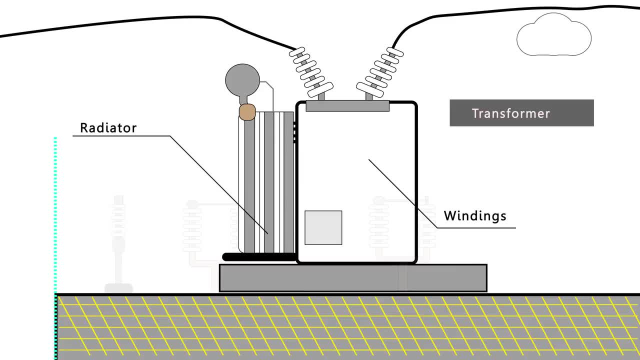 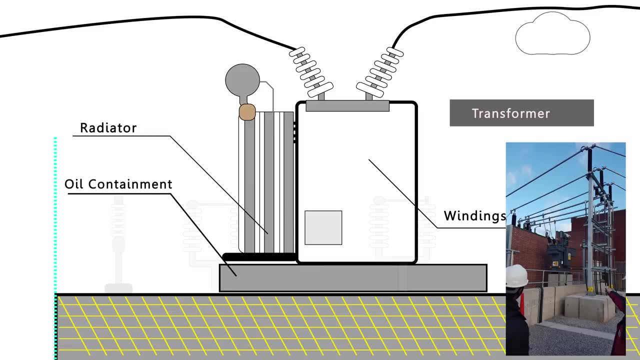 a noticeable feature is an oil containment measure. So transformers contain lots of oil And if they leak there has to be a way to contain that oil. So normally an oil containment measure. Sometimes these are called buns. They're used to contain. 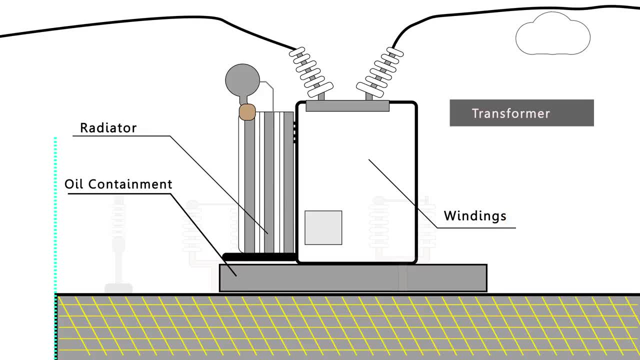 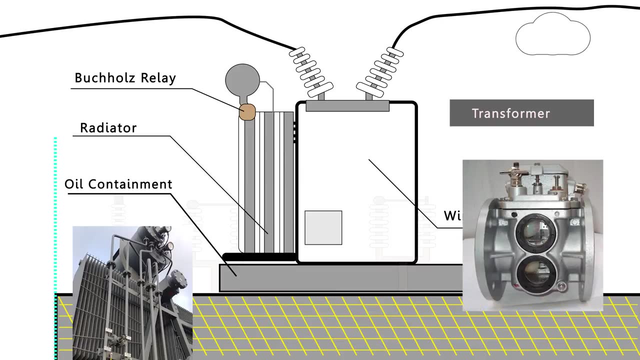 any leak of oil. Now on the protection of the transformer. when the transformer fails, normally you get a reaction in the oil which causes the level of the oil to fall. So a Buchholz relay is a very cheap and effective way to monitor this and to detect a transformer failure. So you'll always see a Buchholz relay. 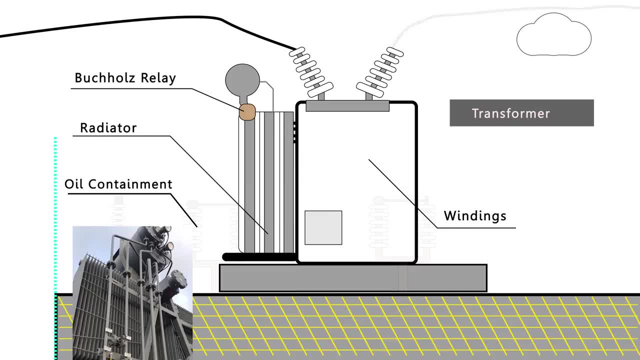 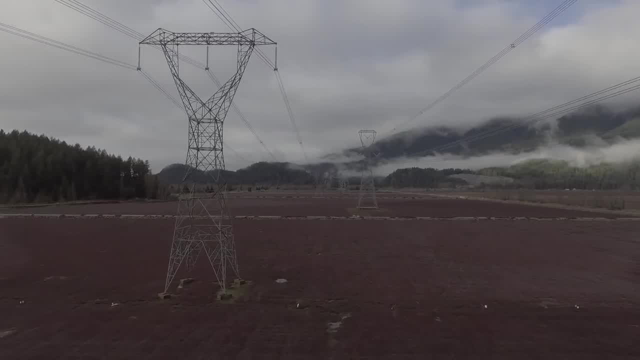 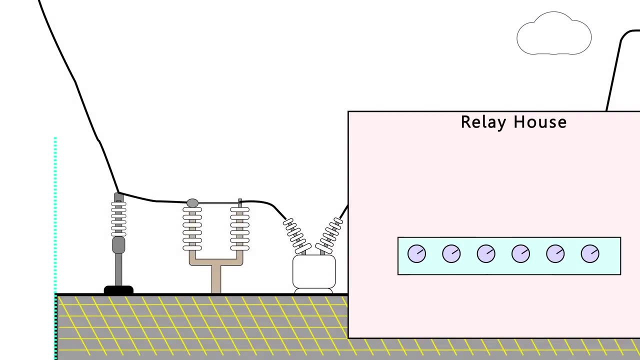 on a transformer. It's just a way to detect failure in a transformer in an automated way. We also have in a substation a building called the relay house And, as the name suggests, this is home to the relays. Of course, the job of the relay is to monitor the 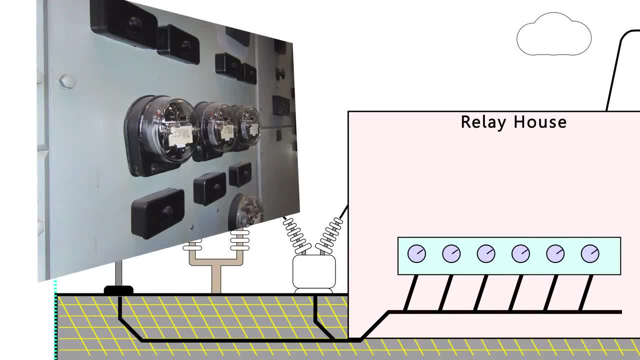 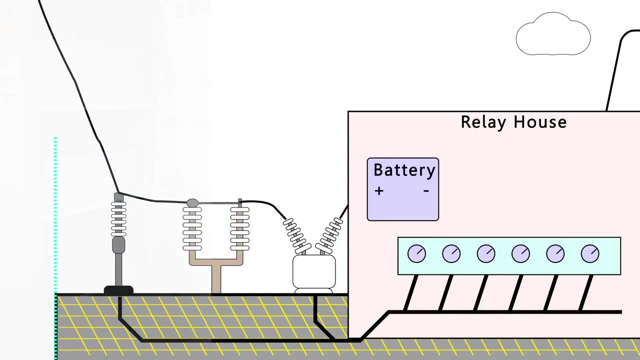 voltage and current and make a decision on whether there's a fault. If there is a fault, it will send the signal to the circuit breaker to trip. So the relay is an automated way to do this. We also have the battery, So the battery in the substation is a way to power the equipment. 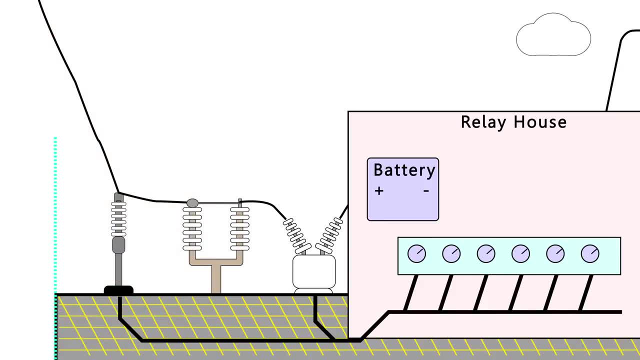 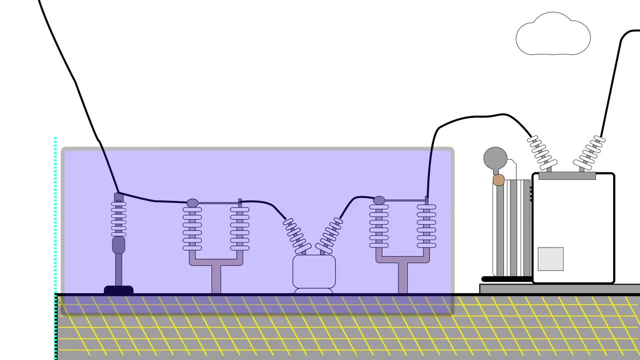 if you get complete power outage. So really important. The battery is so important in a substation And we can group together the VT and CT and the circuit breaker and call these the protection system of the substation. And they perform a really important job in the substation because they actually protect the grid.